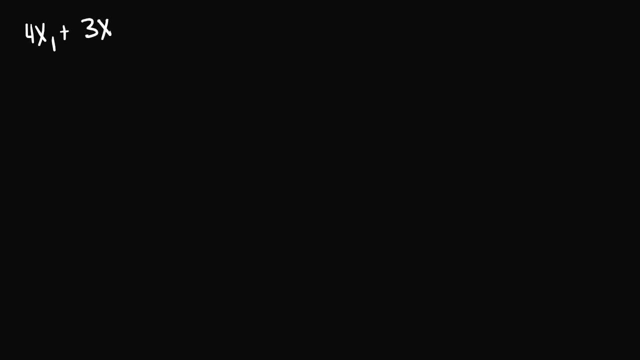 is going to be: 4x1 plus 3x2 is equal to negative 2.. And the second equation I'll just write over here: 3x plus 7y minus 10z is equal to 4.. So these are both linear equations. 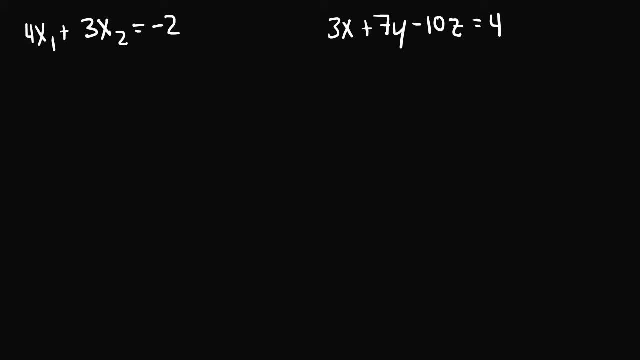 But what makes them linear? There's two important things in both of these equations that do make them linear, And the first one is that none of the variables are raised to a power other than 1.. So in the first equation, our variables are x1 and x2.. And in our second, 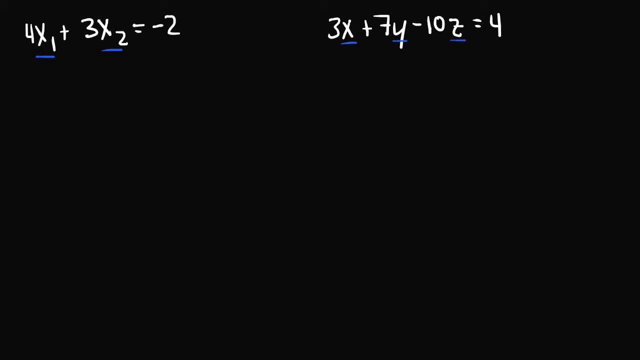 equation. we have x, y and z, All of these variables. these five variables are raised only to the first power. So none of these variables are raised to the first power. So none of these variables are squared, None of these variables are radiated, None of these variables are quad throttle. 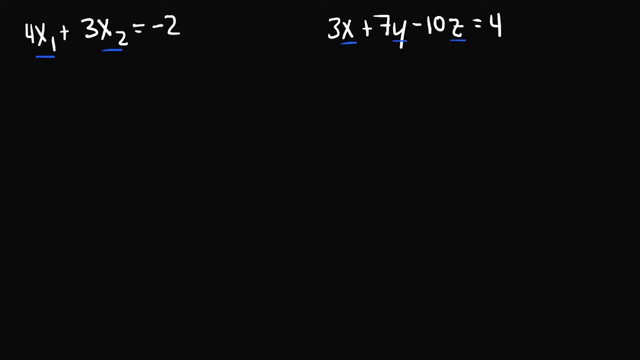 They are not raised to any other power except 1.. If you have a fraction in any of the terms, there should be no unknown variables in the denominator. So if we have an equation such as 3x1 plus 7 over 4x2.. Now, if you have a, 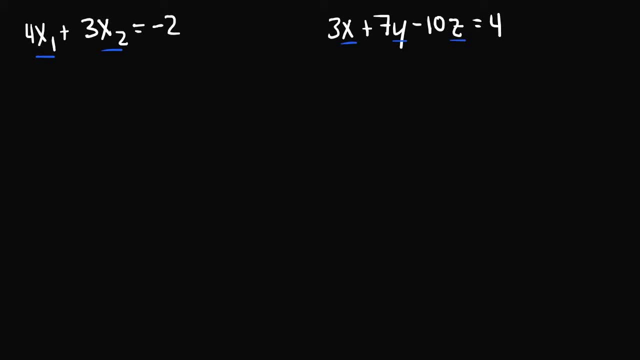 fraction, then that's was the second thing. So if you have an equation such as 2x2 plus 7 over 4x2 plus 2x2.. And if, as this reading, you have a fraction and you have an derivative, 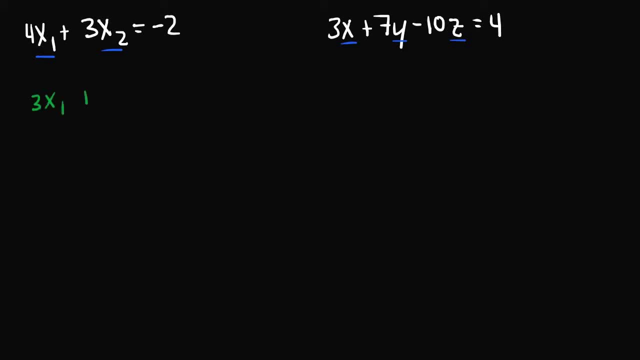 then the games are going to be higher limit than the real term. So that section you can put at the end of the equation. If you want to know, if you can cut the ribbon along the board and then start adding theN gleichgeist equation, then you can fighters, your 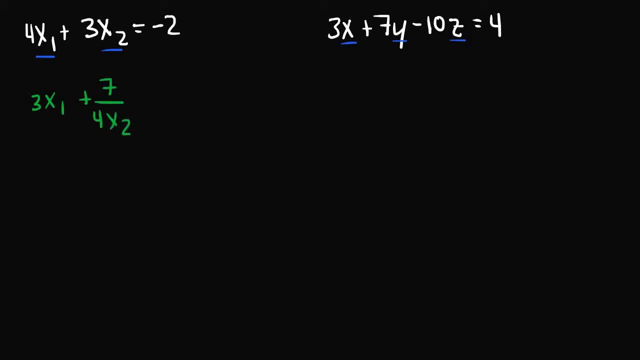 directions, 4x2 is equal to 0,. this equation would not be linear, because you could rewrite this equation as: 3x1 plus the coefficient 7 over 4 times x2 to the negative 1 power, and that's equal to 0. 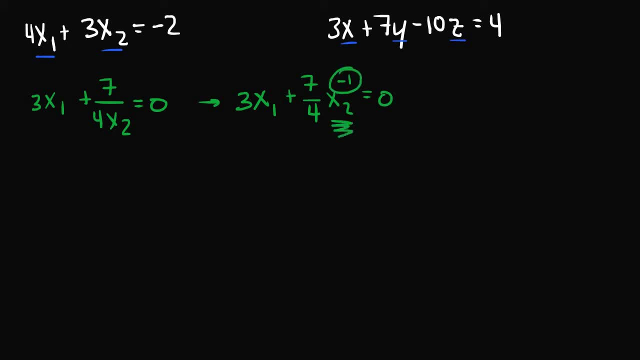 So here we have a problem. The variable x2 is raised to the negative 1 power. So since x2 is raised to something other than 1, this power makes this whole equation non-linear. A general linear equation is just a1 times x1 plus a2 times x2, plus dot dot, dot an times xn. 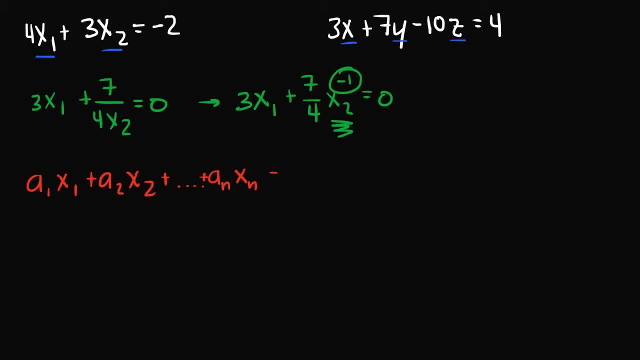 There should be a plus sign right here, right, And this is equal to some value on the right hand side. We'll just call it xn. So in this equation we have a lot of unknowns. In fact, we have an n number of unknowns. 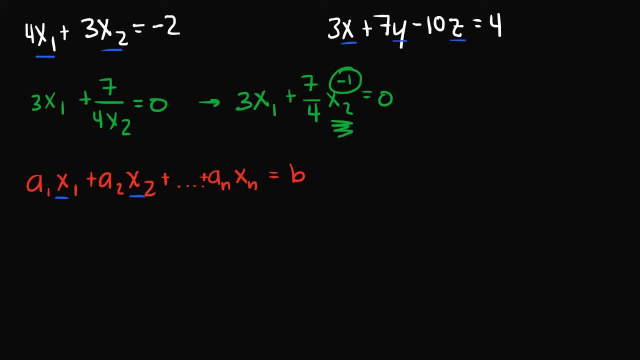 We have x1,, we have x2, x3, x4, all the way up to some xn, And this is equal to b right. So all the unknowns are all the x terms And all of the knowns. so the values that we know are a1, a2, a3, a4, all the way up to an. 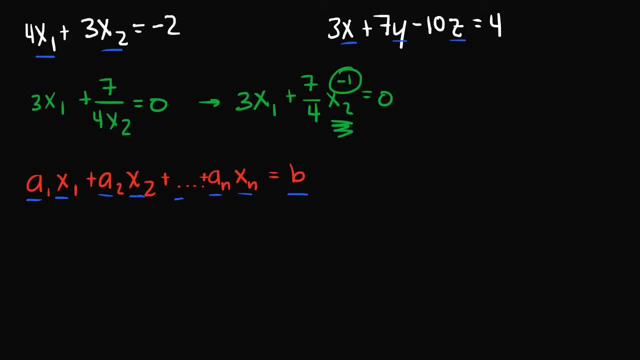 as well as b. We know the value of b. So if we wanted to find something called a solution set for this equation, then we would need to find some set of numbers that satisfy this equation right. We would need to find values for x1,, x2, x3, all the way up to xn. 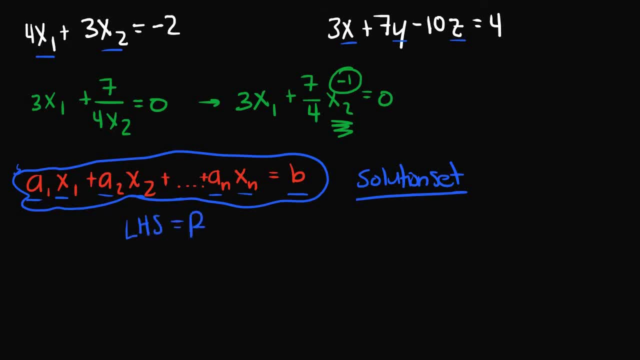 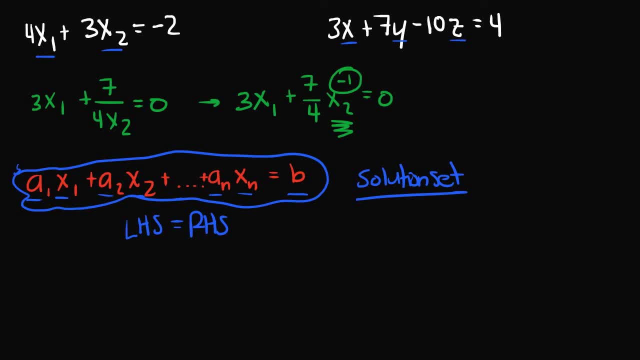 So that the left hand side is equal to the right hand side. So that means that if we found values p1, p2, p3, all the way up to pn, and if these values made sure that the left hand side equaled the right hand side, 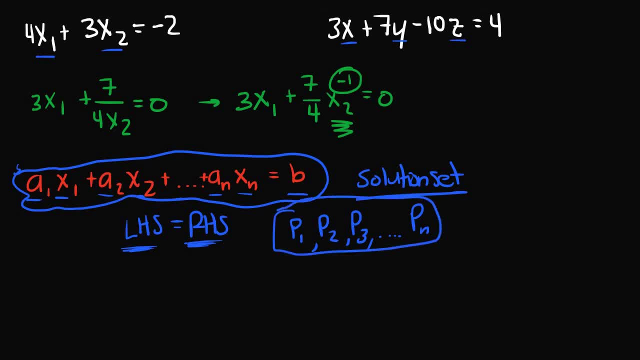 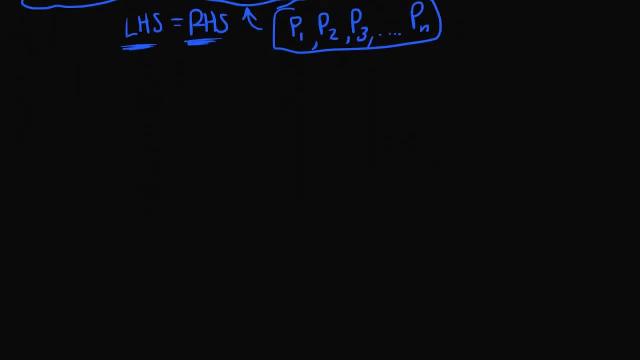 then we would say: all these values p are a solution set to this equation. So we could do a little example to kind of solidify our understanding of linear equations in its most basic sense. And I'll do this in green, I'll just write example up here. 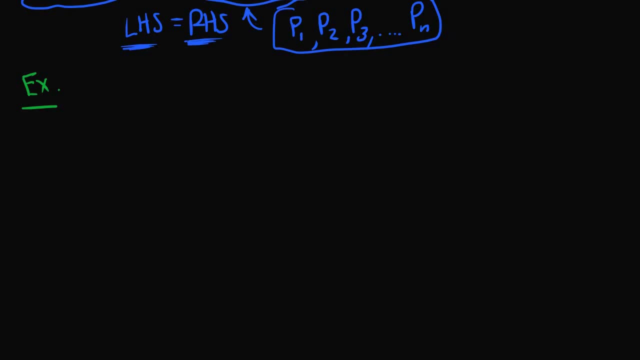 Let's say we wanted to find the solution set for this equation: 3x1 minus 2 over 5 times x2 is equal to negative 2.. So, since we only have two variables- x1 and x2, and only one equation, 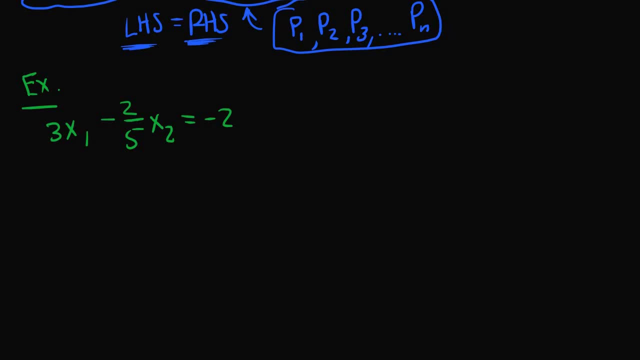 what we could do is we could solve for one of the variables in terms of the other. So let's just solve for x1 in terms of x2.. The very first thing we could do is we could add 2 fifths x2 to both sides.